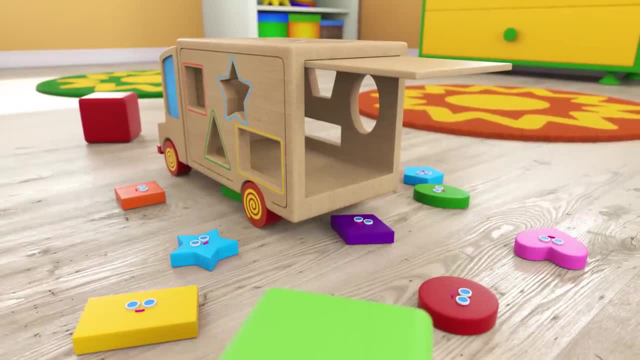 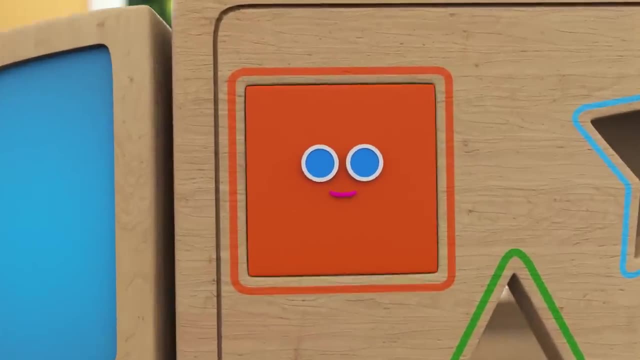 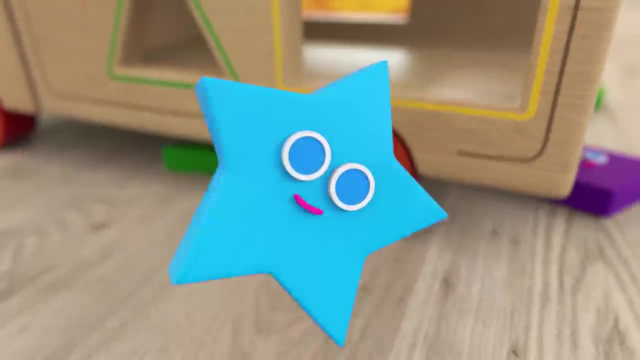 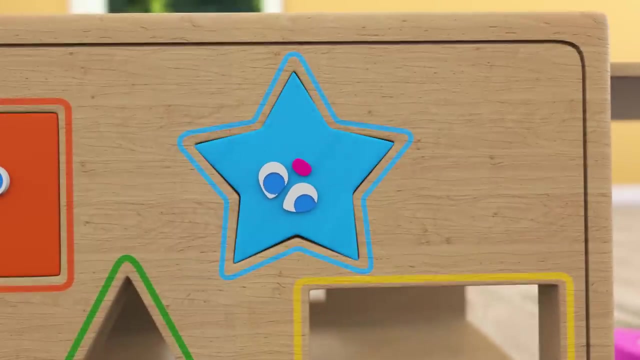 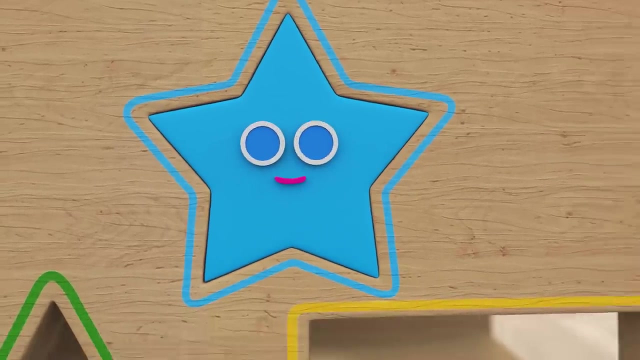 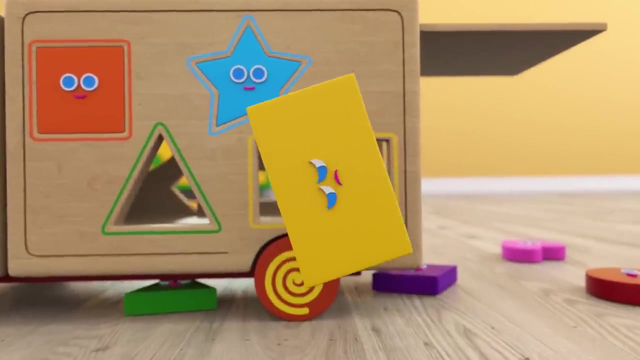 Repeat the names after me. An orange square- Well done, Look, The square has found its place quickly. A blue star: No, This is the wrong spot. Now turn Great. A yellow rectangle, A yellow rectangle. Hey, Turn around. 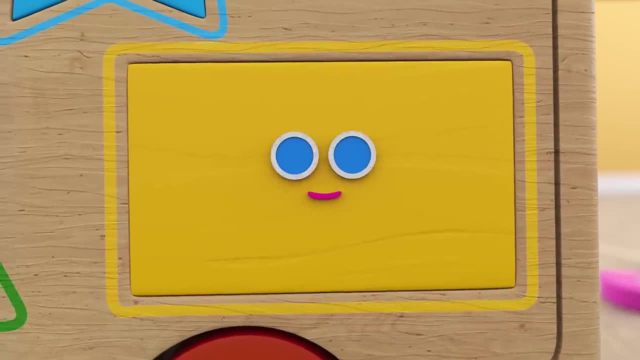 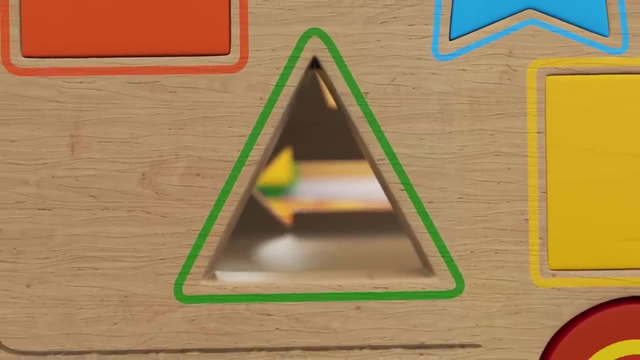 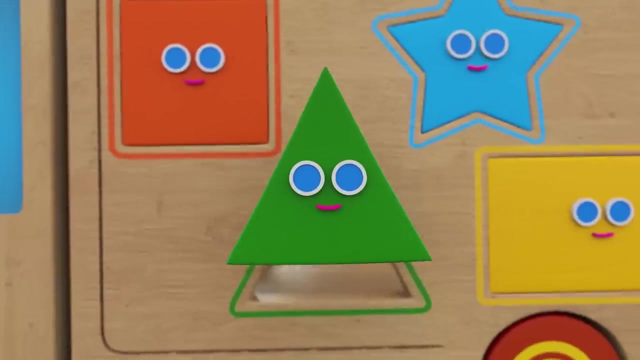 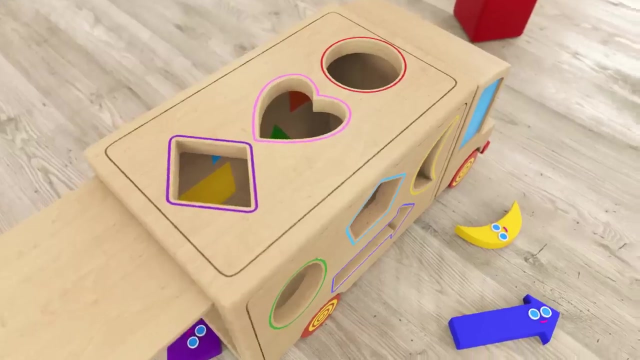 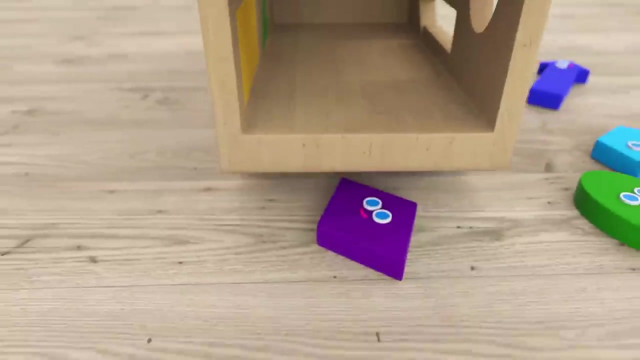 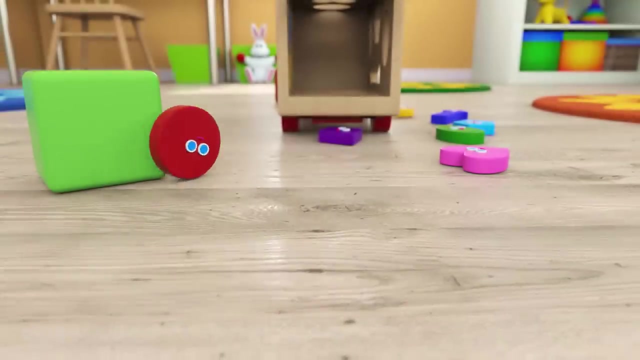 And now everything is well. Look Who's missing here? Hmm, Is it a triangle? Let's look for it. There it is Hiding under the truck. A green triangle, Great. A red circle, A restless circle, is feeling dizzy. 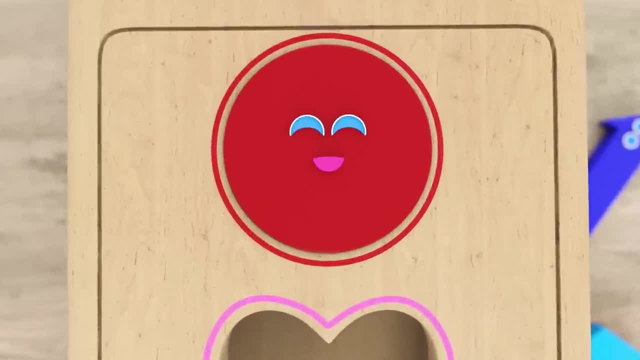 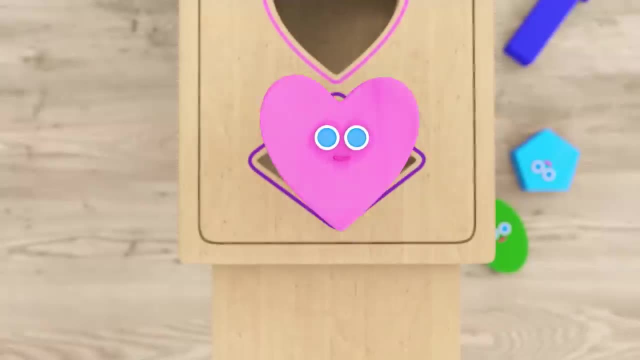 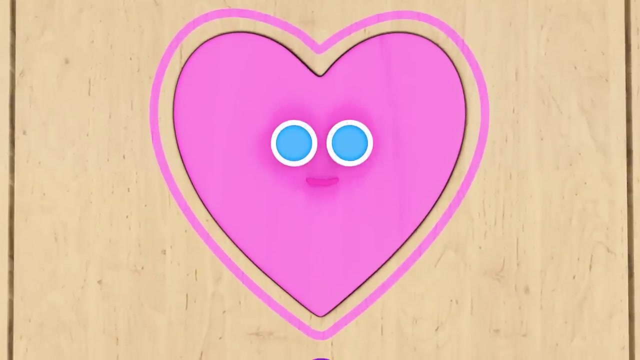 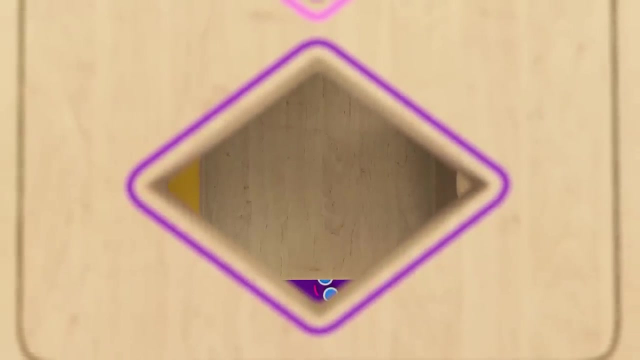 Where is the place for it? Correct, On the top. A pink heart? No heart, It's not your spot. Here's your spot. Oh, someone's missing again. Do you think it's a diamond? Correct, There it is. 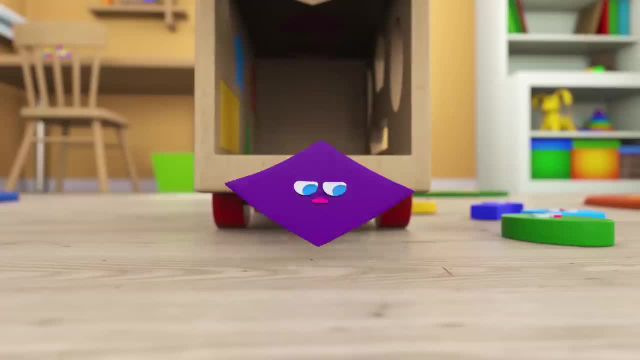 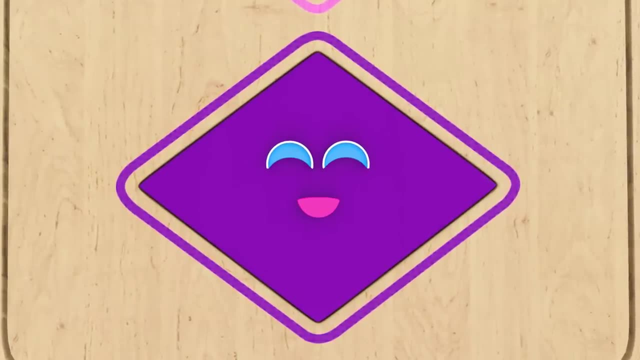 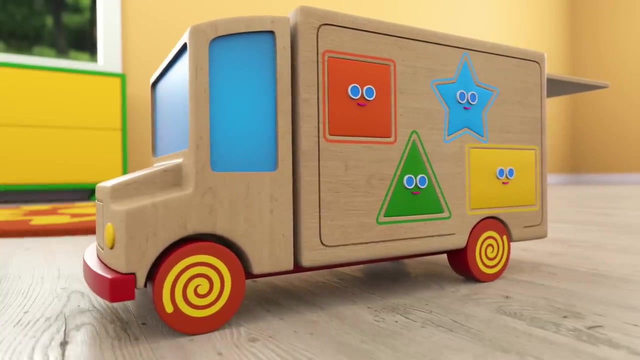 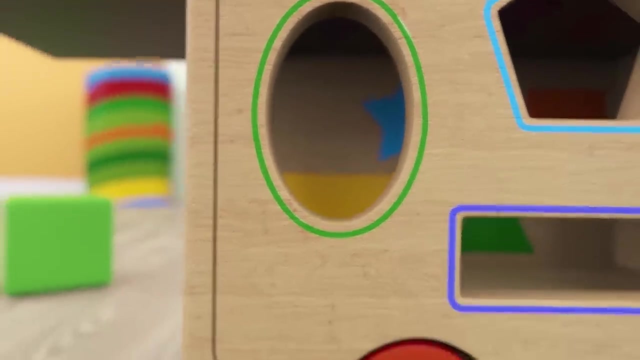 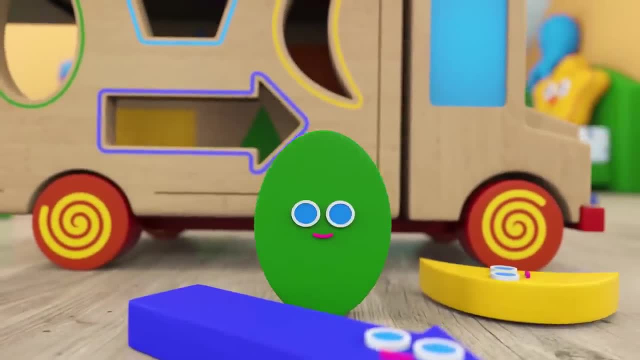 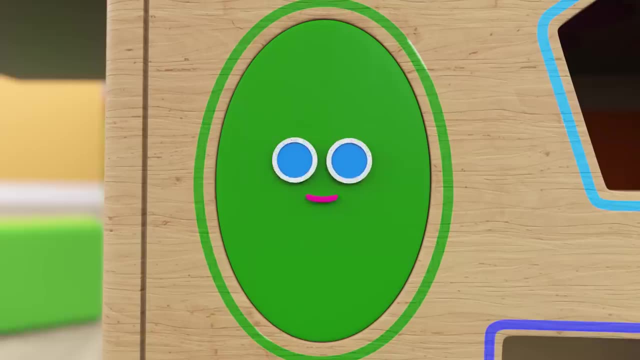 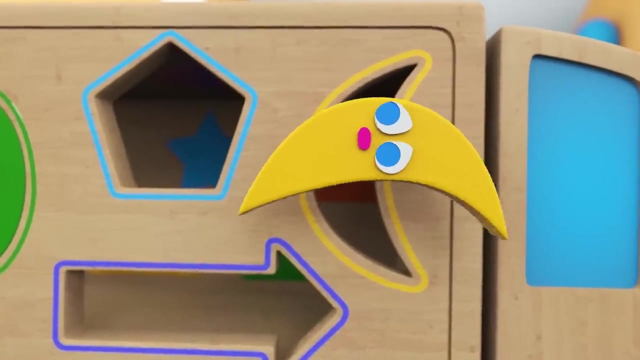 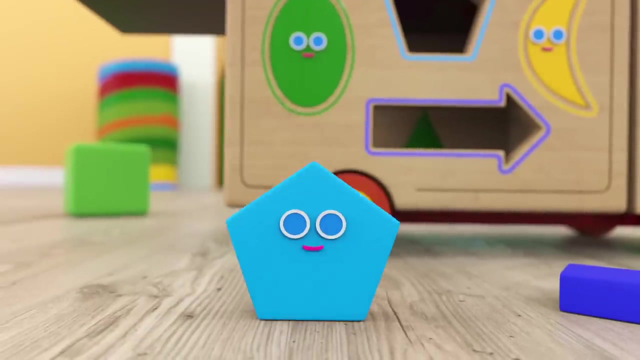 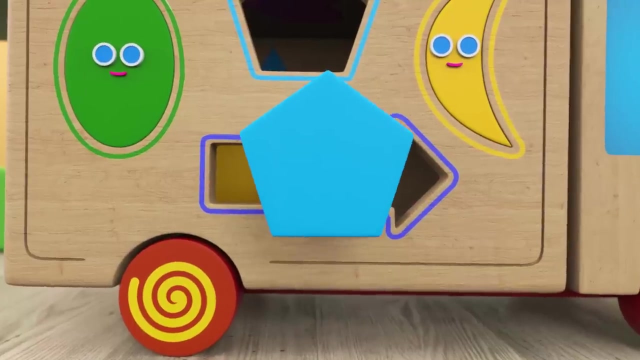 A green oval, Boisterous Oval, Don't hurry up, There we go. A yellow moon, And the moon has also found its place. Great, A blue pentagon? No pentagon, This spot is for the arrow. Come on, pentagon, you can do it.